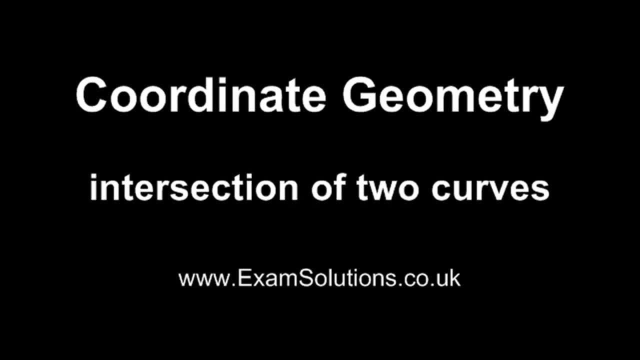 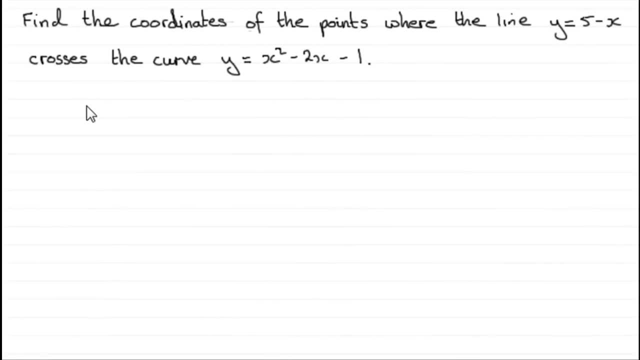 Hi. now in this example, what we've got to do is find the coordinates then of the points where the line y- equals 5 minus x- crosses the curve. y equals x squared minus 2x minus 1.. What I said earlier was that it's always a good idea to see if you can sketch the graphs. 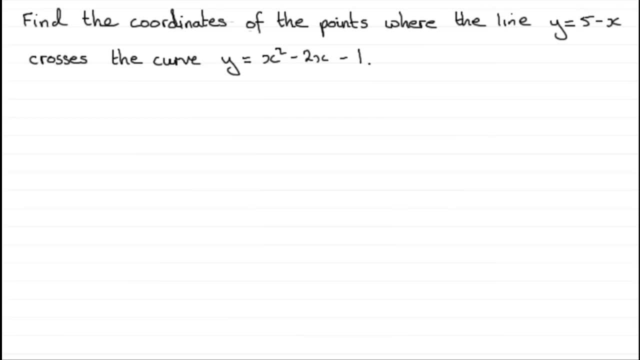 This gives you an idea what your solution should be. And for something like this, we've got the line y equals 5 minus x, which is going to cross the y axis here at a 5, so just mark that in: at 5, got a negative gradient And we have a parabola: y equals x squared minus. 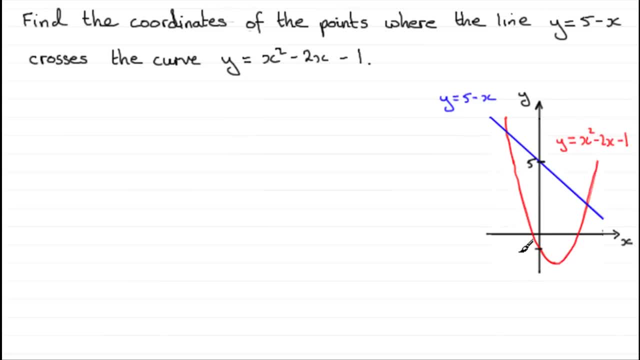 2x minus 1, which we know is going to cross the y axis at negative 1, that's when x is naught And it's going to be slightly pushed to the right of the y axis, that line of symmetry coming through here. 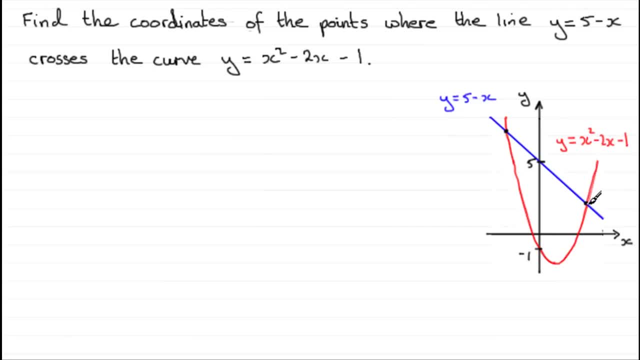 So you can see our points of intersection here and here. So to get those points, what we're going to need to do is solve simultaneously these two equations. So first of all I'd write a subtitle in here: points of intersection, just to give some. 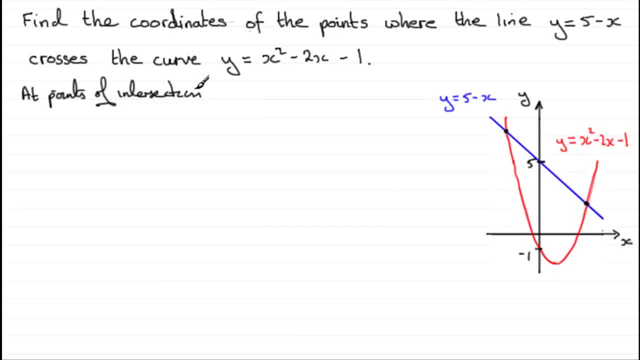 kind of idea I don't know about. many of you have a pat today, but it will be such a brilliant idea to do if you can take an order in your computer like that and say x squared minus 2x minus 1 will equal the value of 5 minus x. 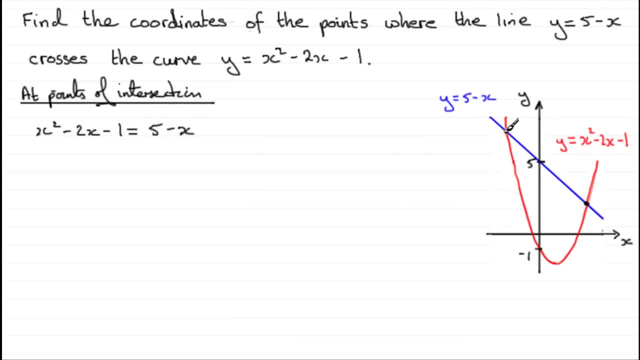 So for some value of x here, the y values on the blue line end the red curve, will be exactly the same, And the same argument applies there, And that's why we can say this: OK, so what we've got here is a quadratic equation, because we've got the x squared. 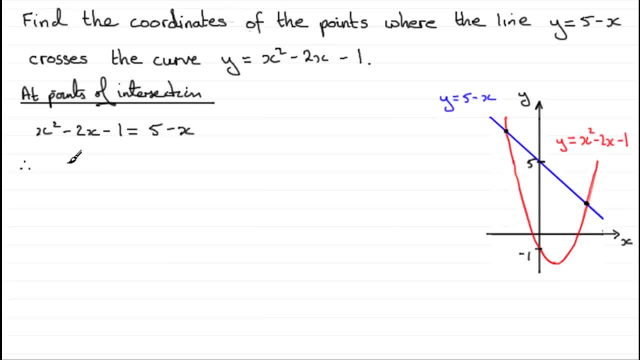 So we need to rearrange it in the form of x squared and then the x term, and then the constant equals zero. So we just need to add x to both sides. So we're going to have x squared minus 2x plus another x. 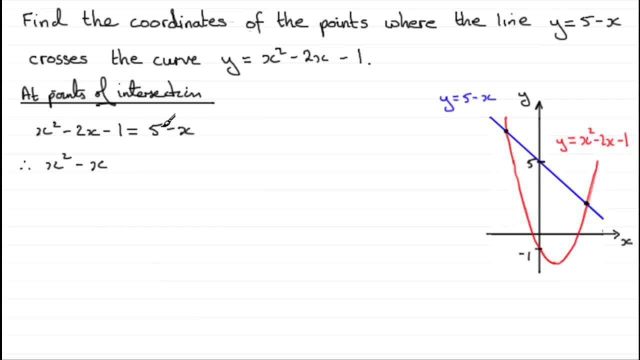 That's going to be minus x, And then we've got minus 1.. And if we subtract 5 from both sides, we've got minus 6 equals zero. So we can either use the formula if it doesn't factorize or if it does factorize, which it does in this example. 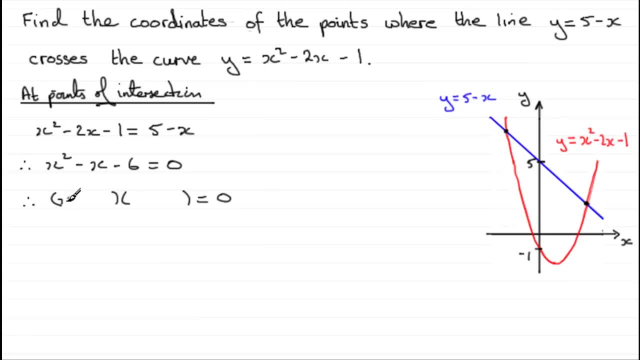 just take the opportunity of factorizing it And what we've got here is x minus 3 and x plus 2.. So each factor would equal zero. So we've got x minus 3 equals zero, or x plus 2 equals zero. 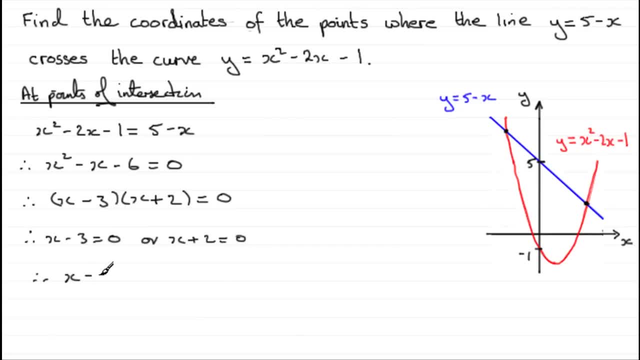 And that would lead to x equaling 3 or x equaling minus 2.. And a look at the sketch here would seem to suggest that this is right. We've got. x is minus 2 at this point here. Let's just mark it in minus 2.. 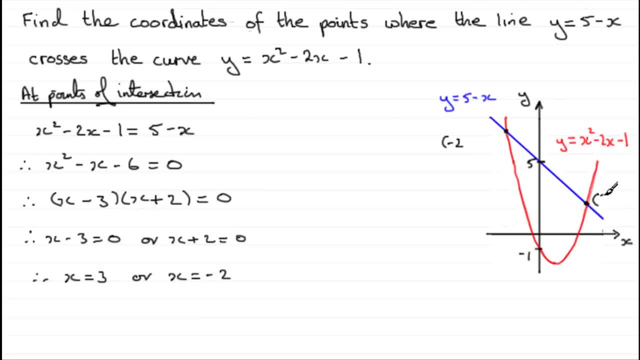 And we've got x equals 3 would be this point over here. Now, what about the y coordinates associated with the x ones? Well, all we need to do is substitute x equals 3 and x is minus 2 into either this equation or this equation. 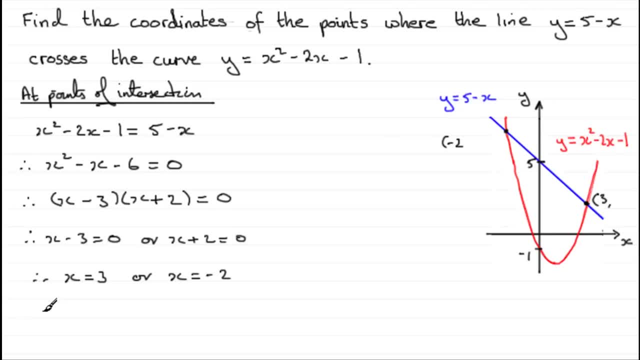 Well, y equals 5 minus x would seem the easier of the two to me. So I'm going to do that. I'm going to say: when x is 3, y will equal 5, take away the 3.. So, 5, take away 3 gives us the 2.. 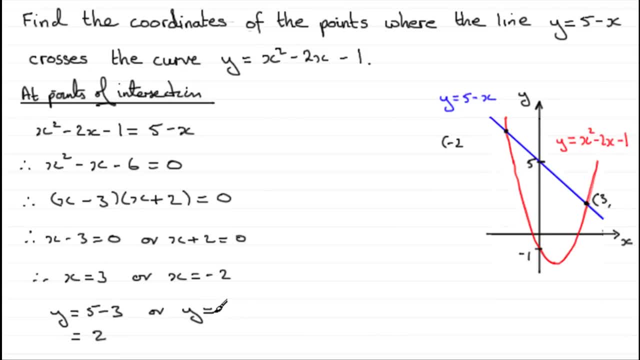 Or when x is minus 2, y will equal 5.. So 5 minus minus 2, and that's going to give us 7, okay, So what we've got in summary, then, is that the points are in section Okay. just wind up the question. 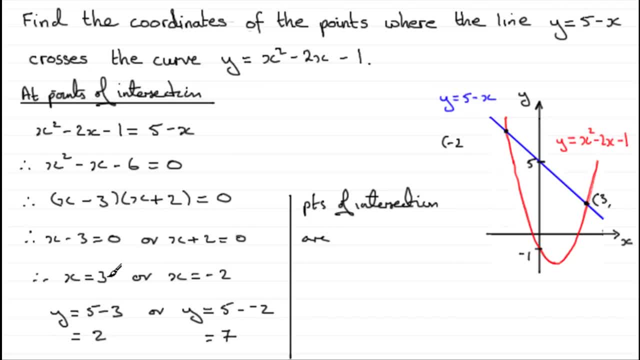 Well, we've got 3, 2 and minus 2, 7.. Minus 2, 7.. Minus 2, 7.. Let's put those y coordinates on. We've got 3, 2 and minus 2, 7.. 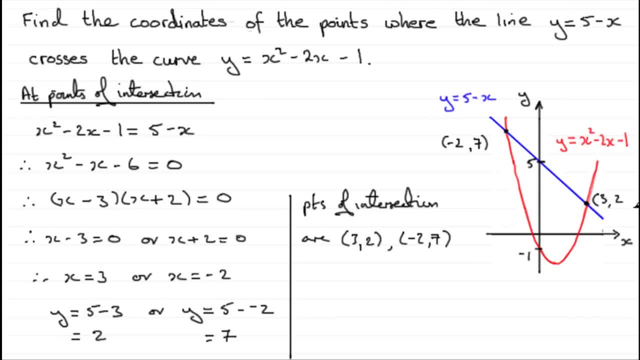 They look sensible. 7 is greater than the 5.. The 2 is less than that 5.. So if I was doing that, I believe I've got it right, But you can always check these back into these two equations anyway.